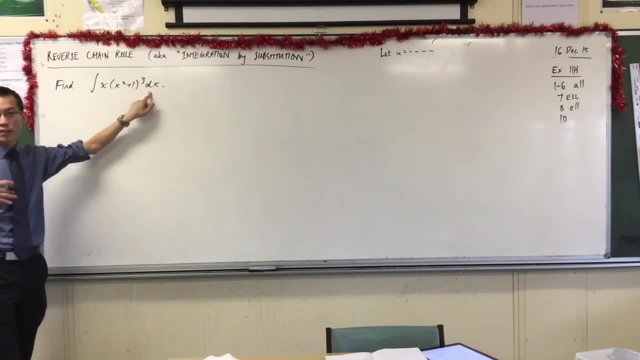 So here's the key: you're going to look in here and you're going to, in this kind of practice, identify what would be a superposition. Now I'm going to choose. I mean, in some ways, it's very obvious for this particular question, I'm going to choose x-squared plus 1, as what I'm going to substitute out. okay. 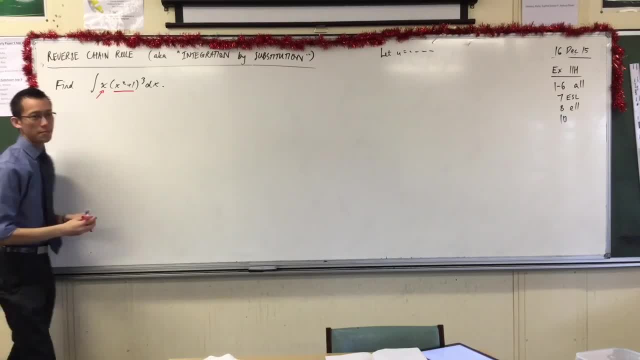 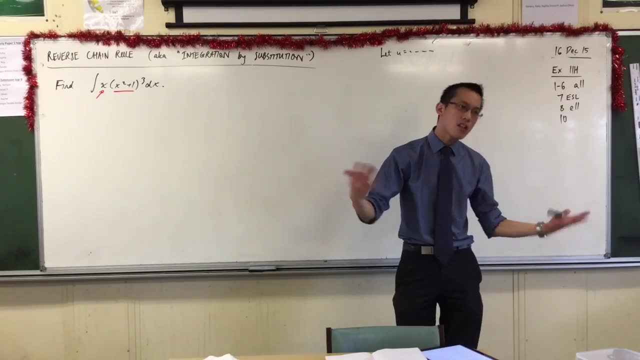 And part of the reason why is because beside the x-squared plus 1, I see x. now x is very, very similar to the derivative of x-squared plus 1, it's not exactly the same, but it's only off by a constant, so it's very easy to work with okay. 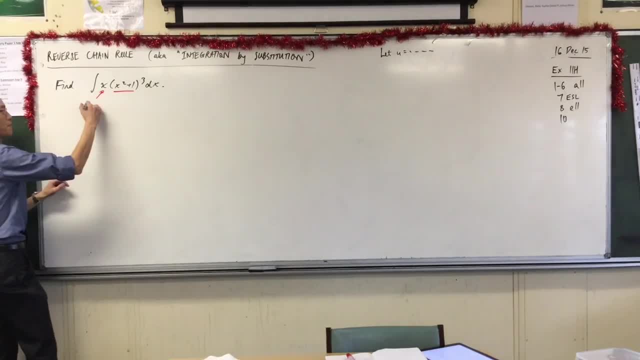 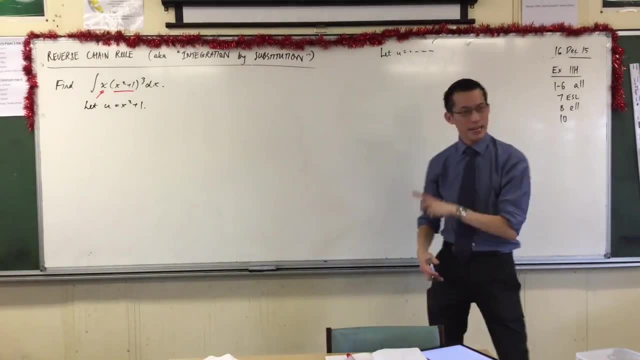 That's right. So what I'm going to do is I'm going to say: take that guy and let's replace that with u. Now, if I'm going to change that variable- that kind of changes everything, because you can't just put u in there- Then you're going to have x's and u's and a bit. 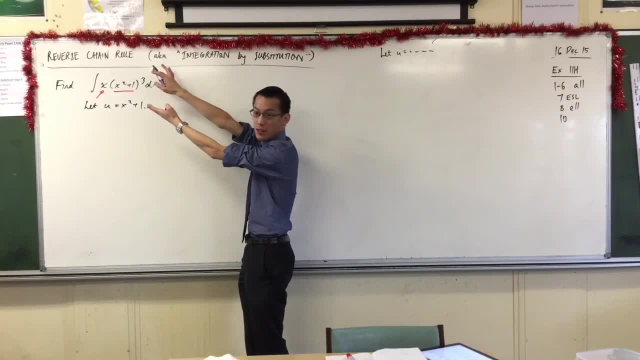 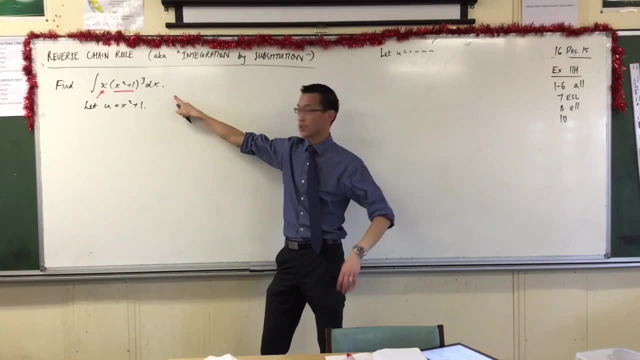 of a disastrous mess. If you have it all in x's, that's okay. If you want to go to u's, you've got to go all to u's. So I'm going to have to change this and this and this. Here's how I'm going to do it. See how I've got a dx there. That means differentiation. 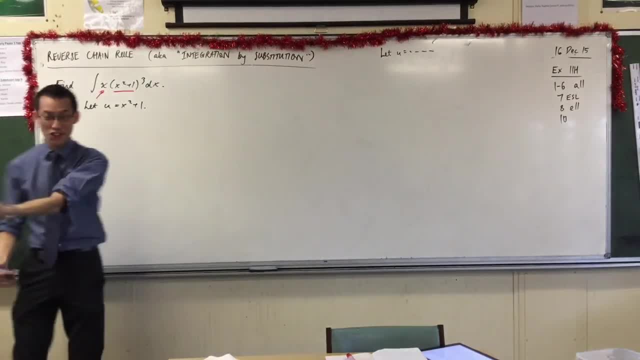 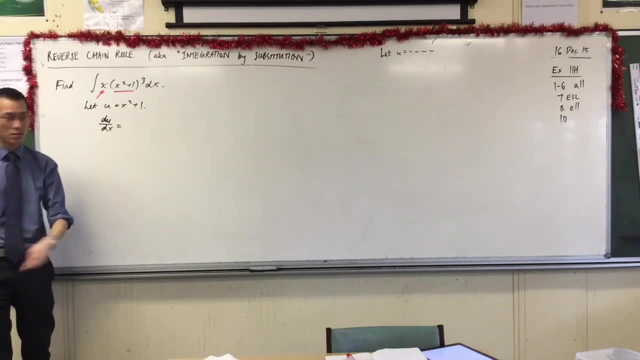 or integration. So if I take u and I differentiate it, du on dx, So I'm differentiating this with respect to x, What is the derivative? Just 2x. Now I don't have 2x in my integrand. 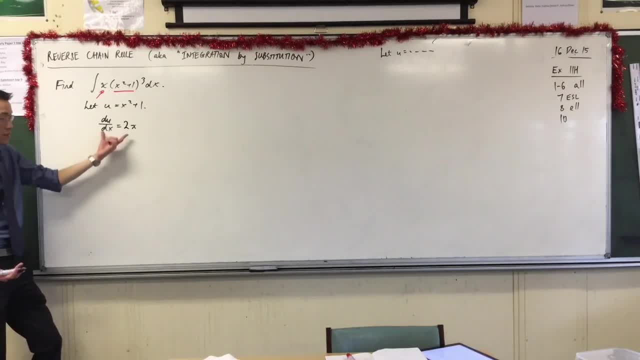 I don't have 2x in my integrand, However, I have x, which is very close to that. All I have to do is divide both sides by 2.. So you can see now, in one fell swoop, you can see here, using this line, here I'm going to be able to eliminate both of these guys. 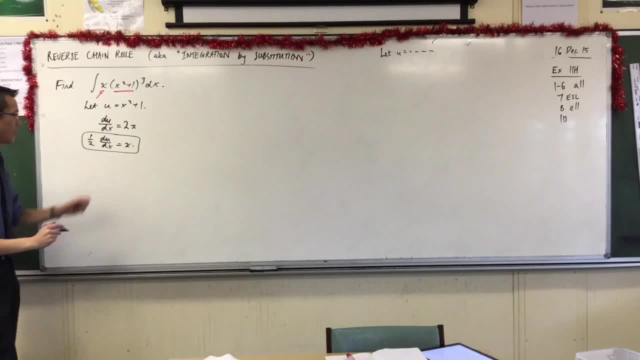 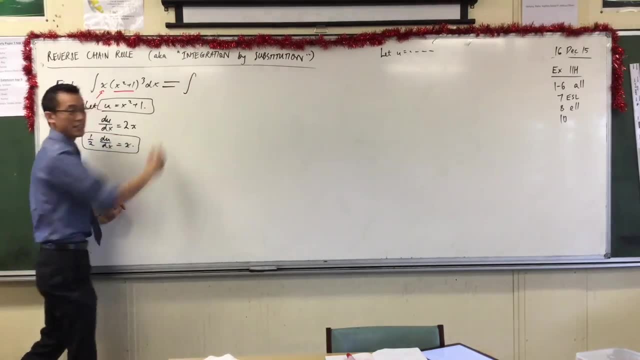 and replace them with their equivalents in terms of u. So now that I know this and this, I can say: therefore: this thing is equal to integral of now. first, I'll replace the x squared plus one. That tends to be the way I do it. This will be my new integrand It's. 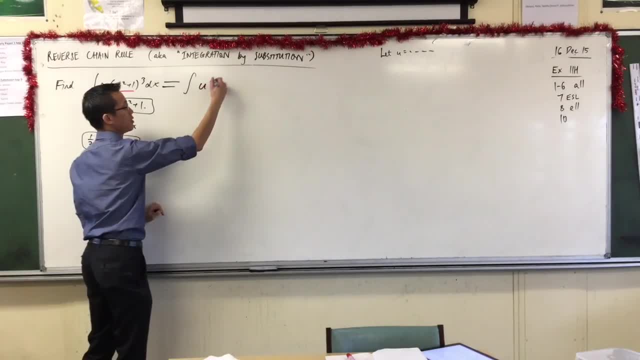 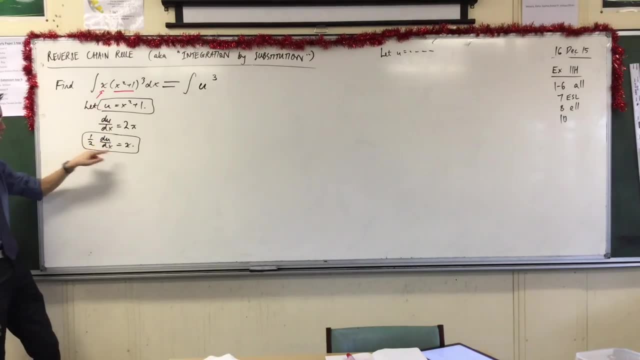 going to be not x squared plus one, but u cubed, There it is. It's gone. Then I do this Here's: replace my X right with this guy right. it's a bit messy but you'll see it quite easily comes out in the wash. there's the X that was hanging out the front and 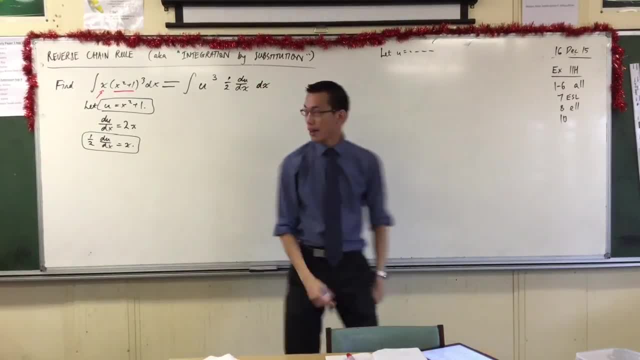 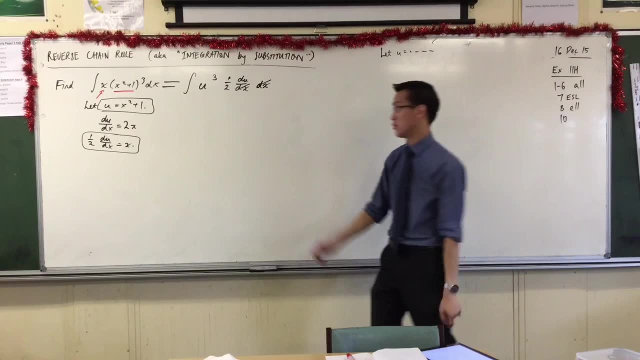 then there's a DX here. okay, now you can see what's going on here. I have these two things canceling. it's just like a fraction, right, like we dealt with. rise over run before we've got divided by run and multiply by run. they'll disappear. 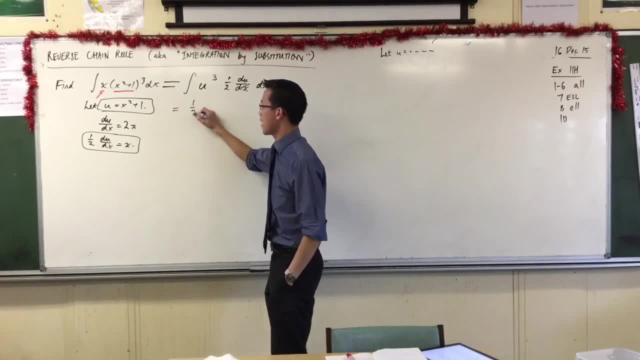 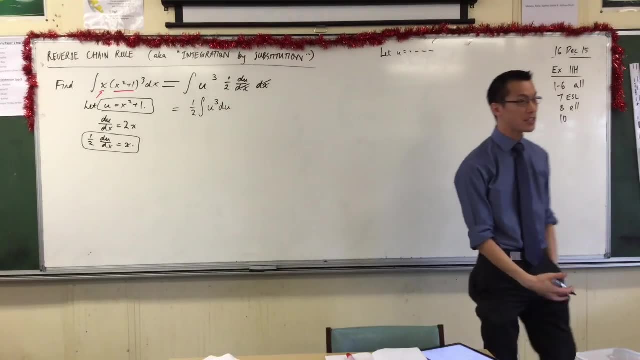 and now you can see what I'm left with is if I take that half out the front just to tidy it up. this is u cubed, do you right? so now I'm integrating with respect to a whole new variable, but it follows all the rules that we know. 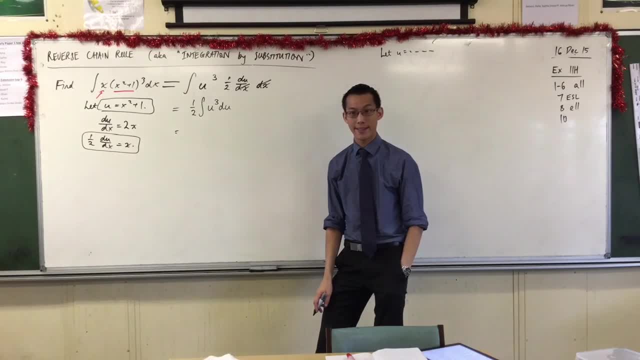 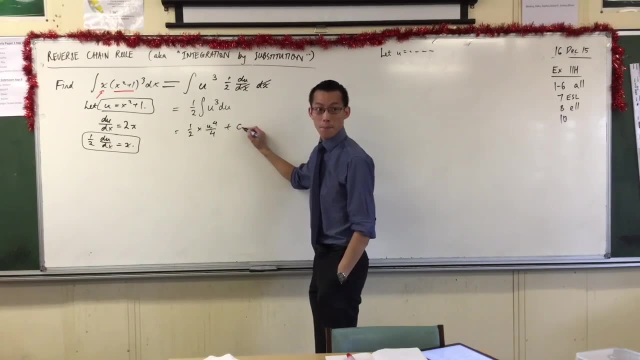 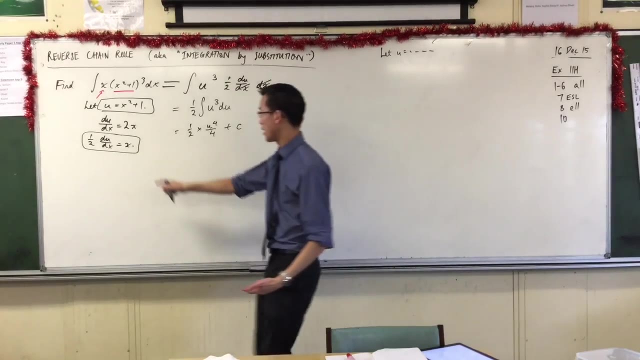 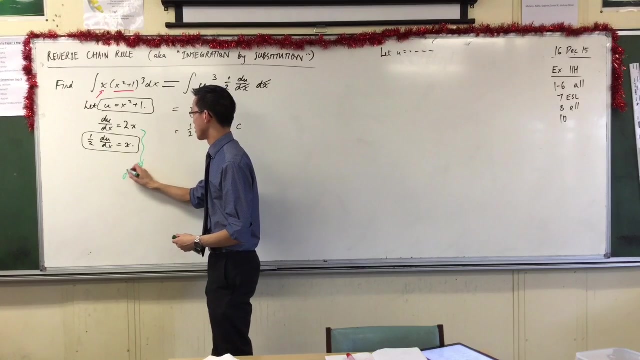 before. right, what's the primitive of u cubed u to the 4 on 4? yeah, wait, where whereabouts make do you the subject? you be here. okay, all right now, some people will do it like that. okay, they'll sort of do this, they'll write. 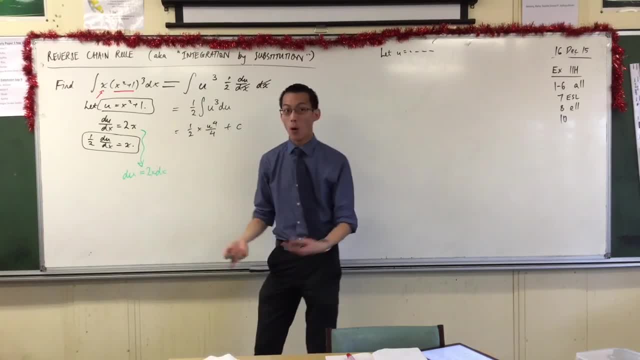 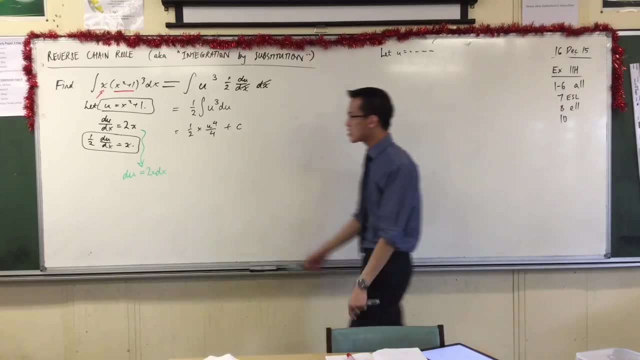 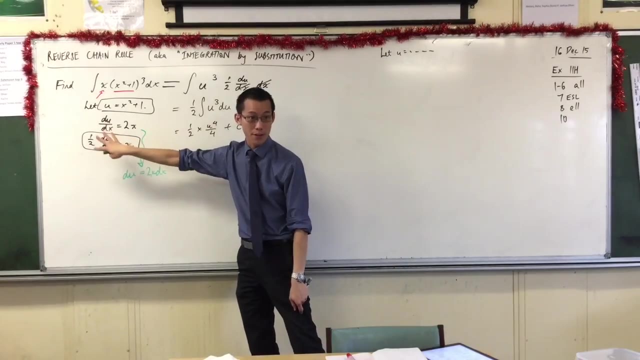 that, something like that, or they'll make DX the subject to get rid of that. either of those now I've seen those before. I think I think they're okay. I think it's a bit dangerous to throw these around just as independent things. I kind of like doing it this way because it shows I got it from a derivative right, like. 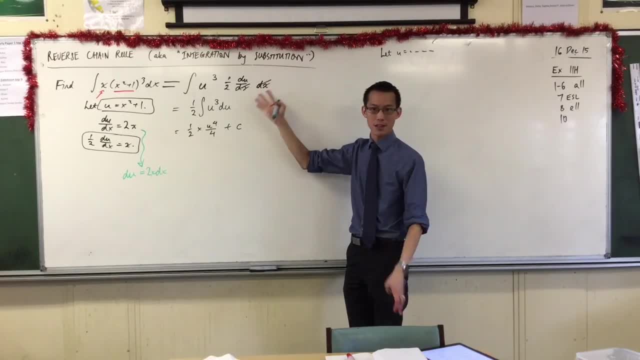 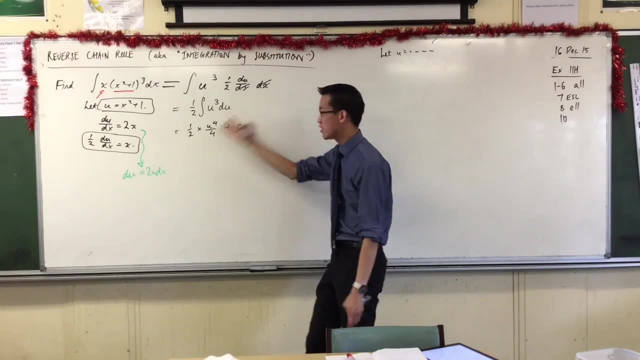 even though DX and DUs do follow a lot of the same rules, as normal arithmetic does, right, they'll sort of follow all of them. so that's why I kind of leave it attached to its DU. as you can see, you're gonna get the same result, it's okay, but um, and I don't frown. 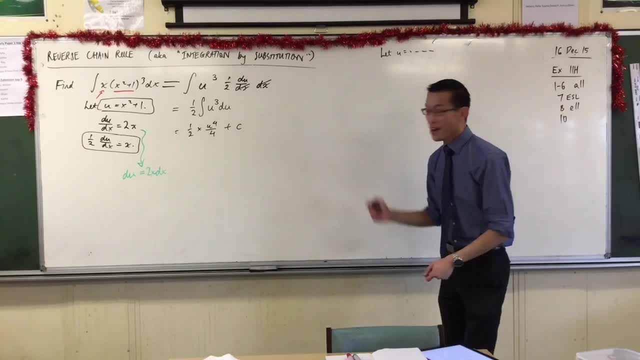 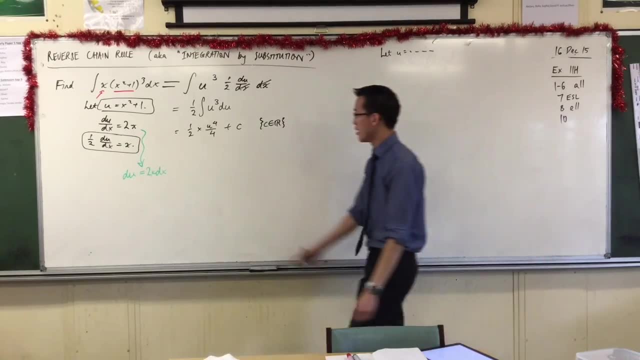 on that, but I do it this way, I do it that way. it's my preference. okay, I've got my constant flying around there. I should say that that's a number, not a. it's a real number, not an actual variable. and then just to tidy up right: 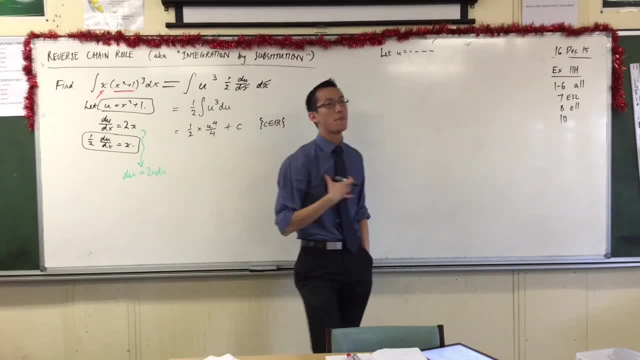 my question started with X's. I introduced you to make it easier for me to solve, but the question has nothing to do with U's. okay, so therefore I've got the 1 over 8 out there front from the 2 and the 4, and then what I'm left with is this: that's u to the power. 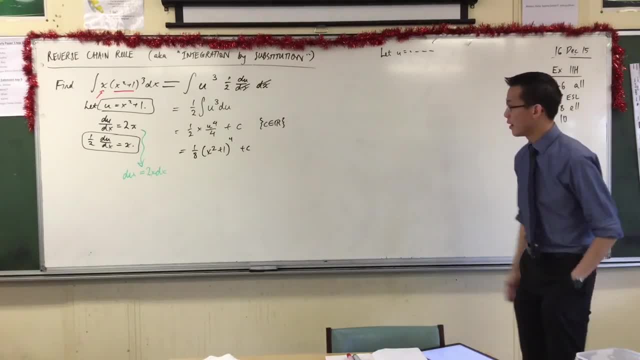 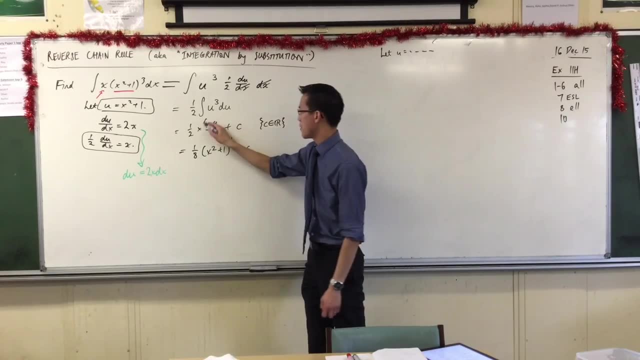 of 4, plus my constant. and I'm finished. And just as a quick note, some of you might have noticed: hey, hey, hold on a second. this half that multiplies by this, shouldn't that mean that the whole thing is multiplied by a half? And it kind of does, but you know. 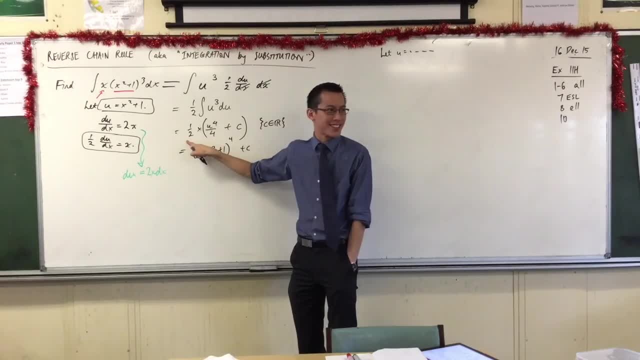 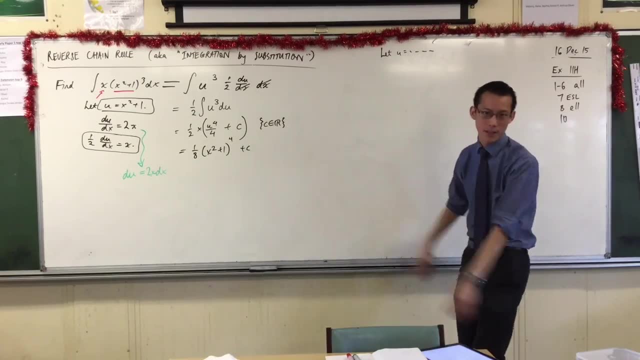 what A constant or a half of a constant is still a constant, right, It's just a different one, and I don't care what its value is at the moment, because it's indefinite. I've got all of the constants just by saying plus c. So that's why, from this line to this line, 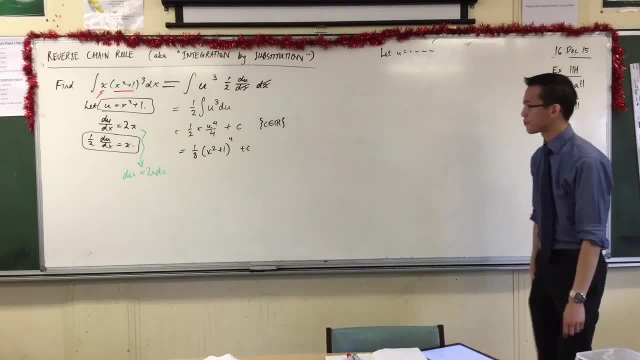 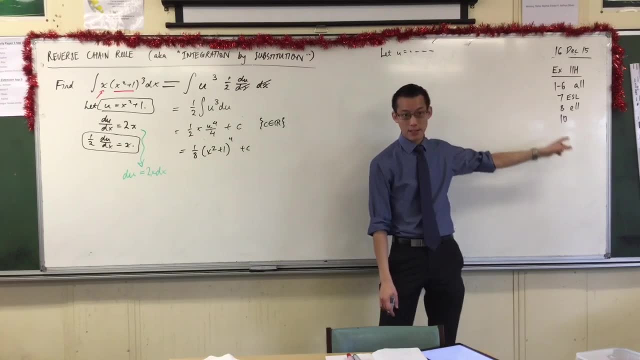 I can be pretty relaxed with that constant. okay, So that's it. It's not complicated. okay, Now, just as a very simple extension, and you won't need it for this exercise. but it sort of begs the question, right, What if I just subtly change the question from: 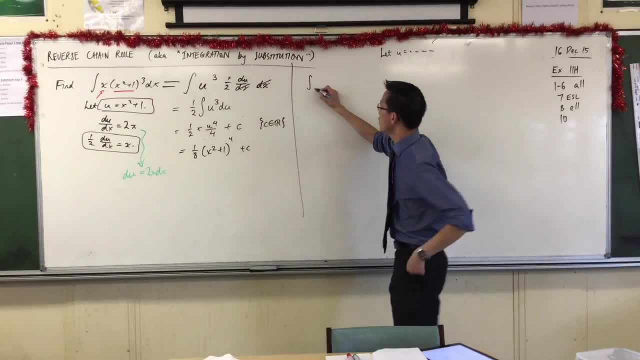 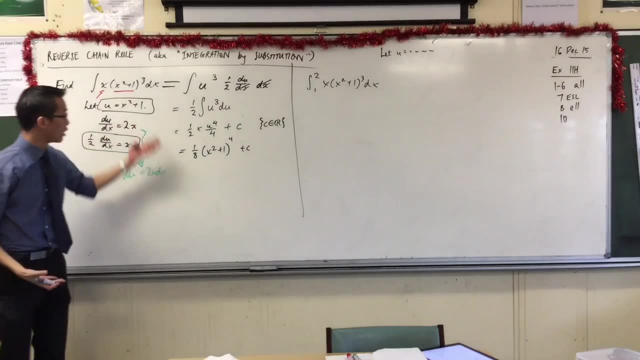 an indefinite integral to a definite one. Okay, now I have some boundaries on this, okay, So obviously, a lot of this is going to play out in exactly the same way that the original question played out. However, remember how I said to you before you translate everything here: it's all in x's, You translate it so. 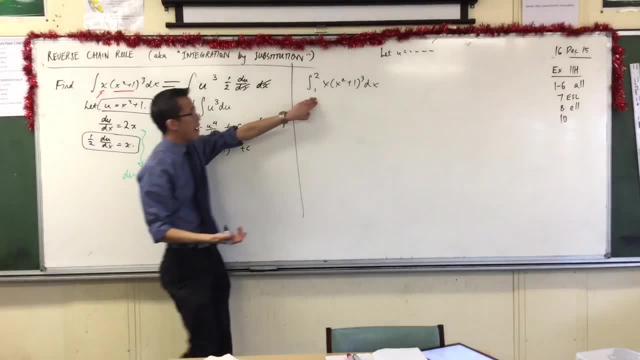 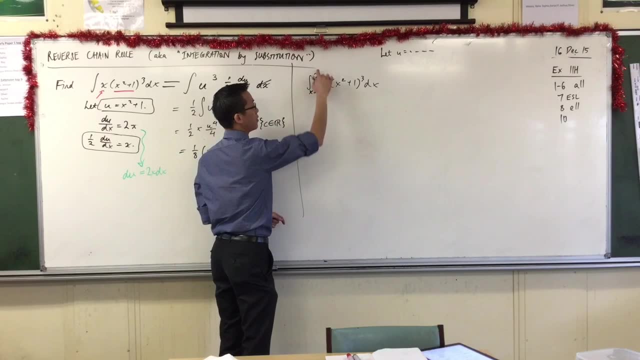 it's all in u's. you see that? Okay. Well, these boundaries, they are x boundaries, right? In fact, the 1 and the 2, there are really shorthand for x equals 1 and x equals 2, okay. 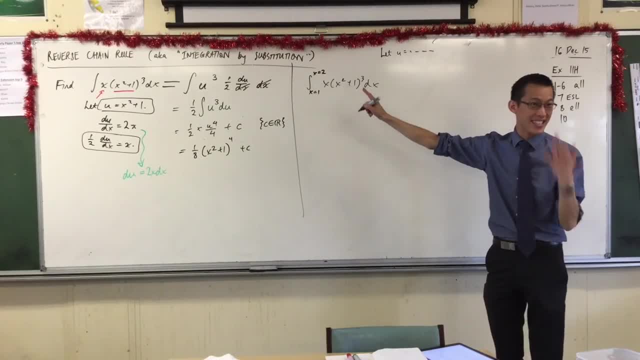 In fact, when I'm doing these kinds of questions, I write that for myself as a signal to say, hey, don't forget, don't forget, you've got to change them as well, right? So I would say, well, if I let this equal this, I'll do all my d1, dx business like I did before. 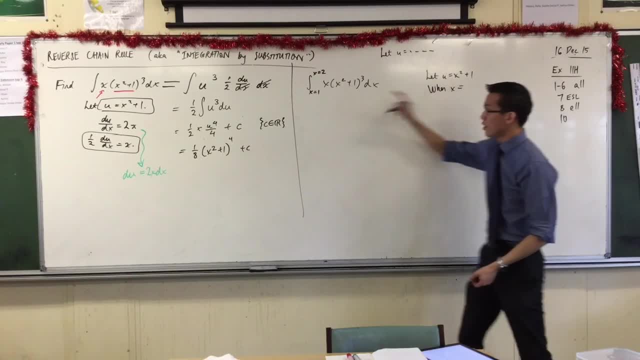 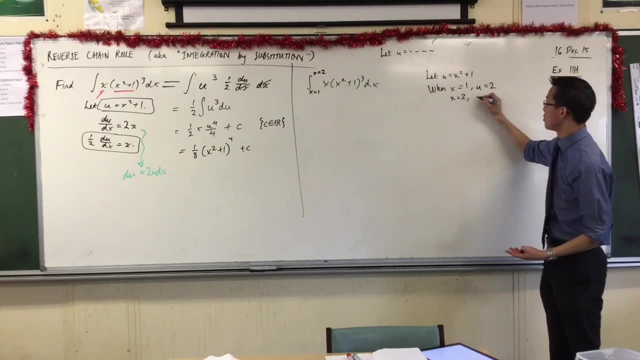 but in addition to that, I'll say: look, when x equals 1, u's equal to something else. In this case, I think it's 2, yeah, And when x equals 2, u's also equal to something else. 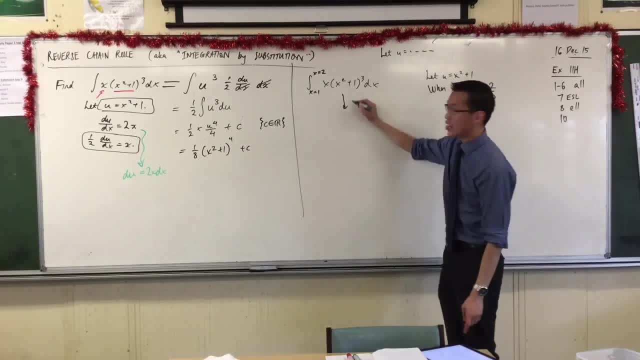 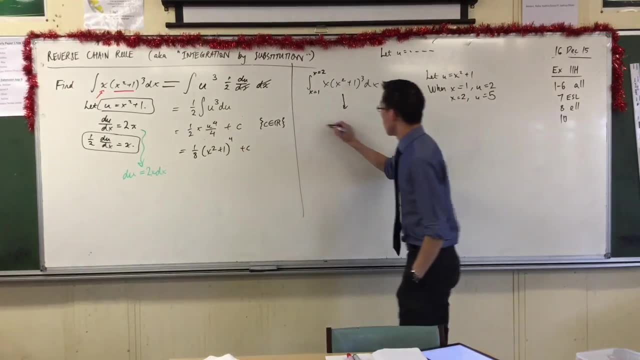 I think it's 5 in this case, right? So when I go ahead and I change the question from this thing to all be in terms of u's right, I think this is what I ended up with before with my indefinite integral right. Well, I'm going to end up with the half and that. 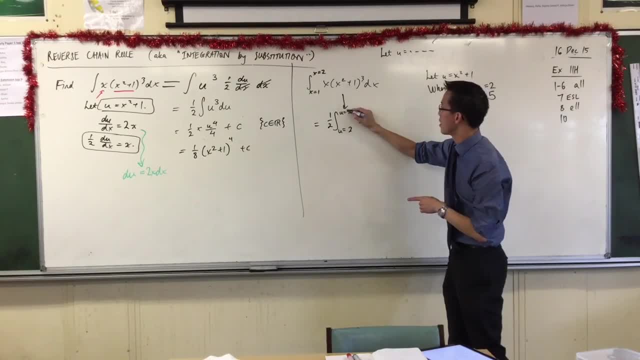 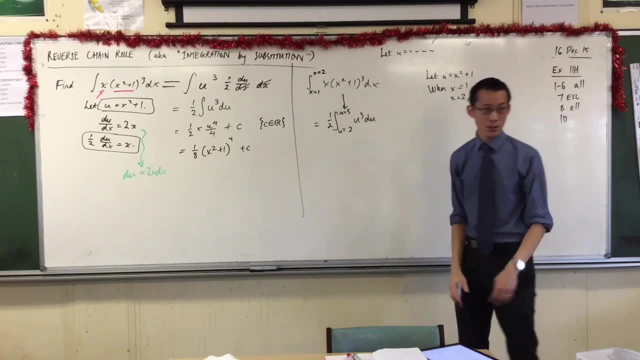 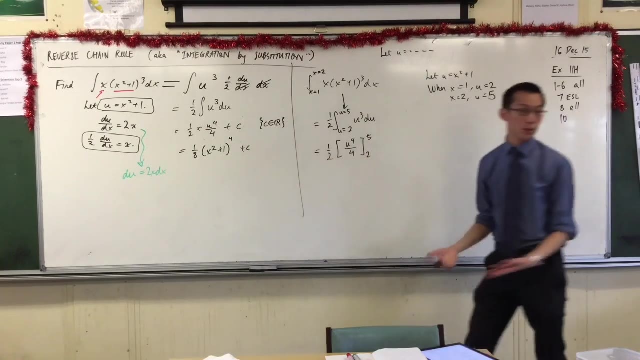 and I'm going to get two brand new boundaries that are u boundaries, not x boundaries. okay, So this will end up with this like. so It will unfold just like it did before, but now I'm going to put these numbers in. okay, Now it's worth mentioning. 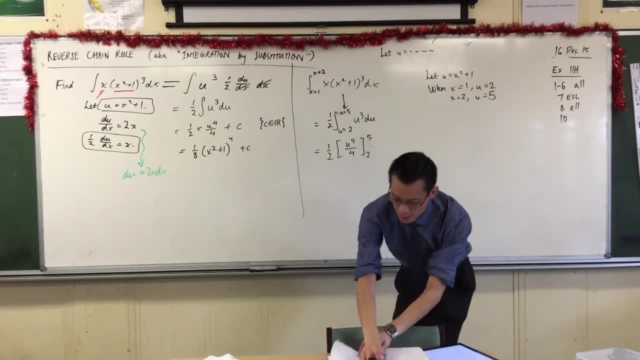 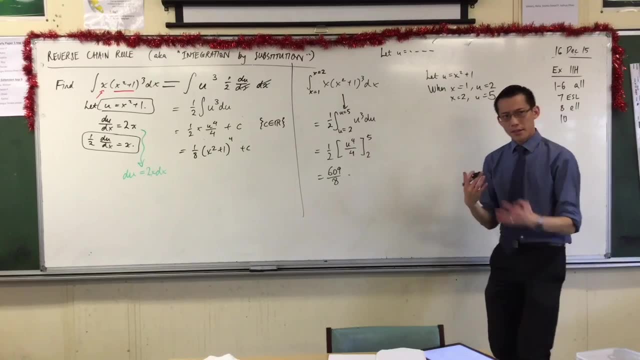 you're going to get. you're going to get a number out of this. I think I've already evaluated this. If I've crunched my numbers right, I think you get this okay And just really quickly. there's a bit of a strange question here in that like why did I have to go back to x here?